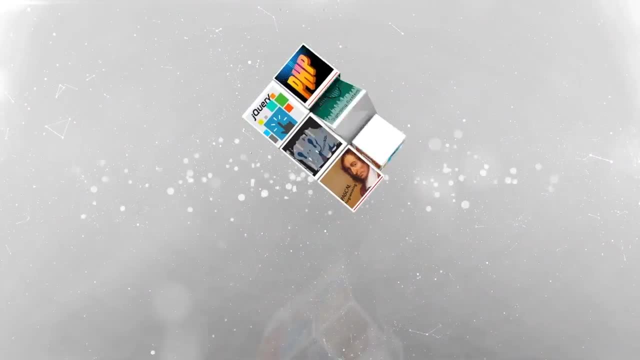 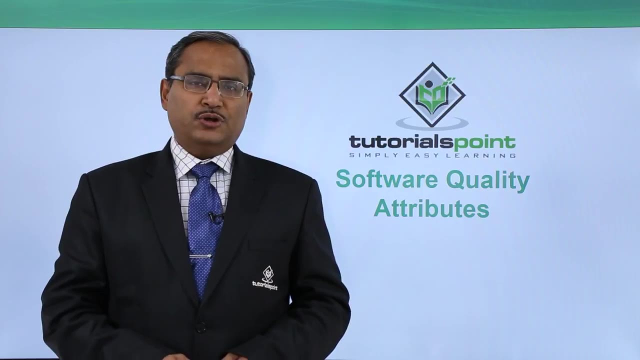 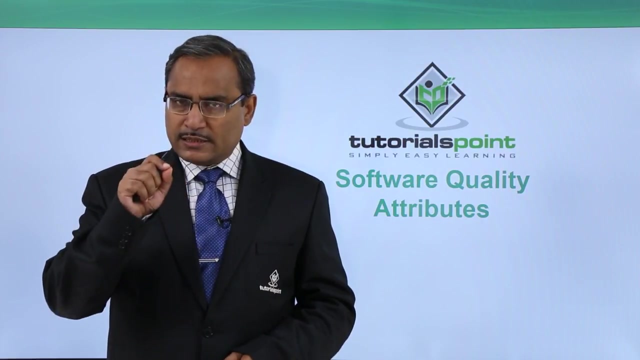 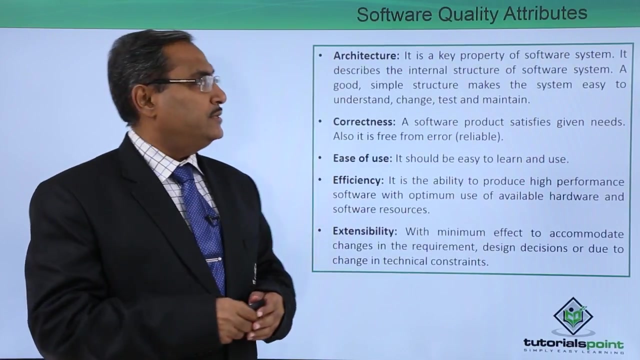 We are discussing software quality attributes. So what are the different attributes which will decide whether this software is a good quality or not? So let us discuss all these attributes into further details. So first one we are going to consider that is our architecture. So it is. 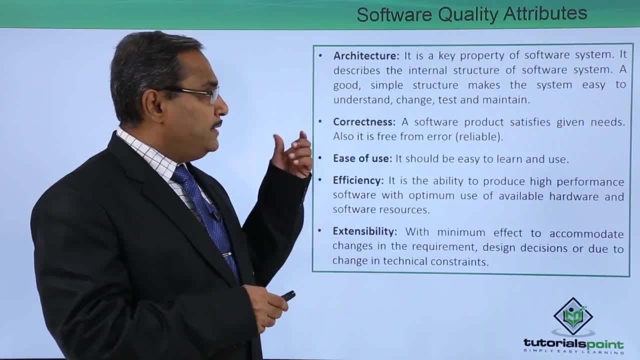 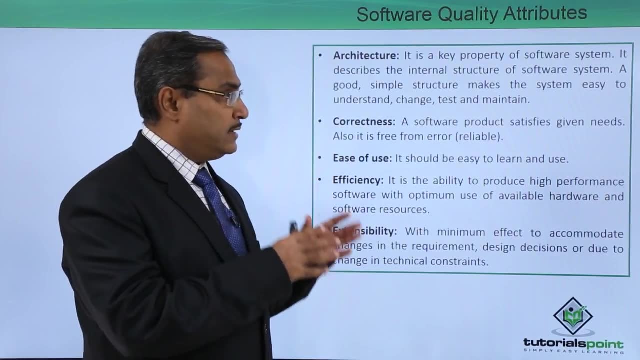 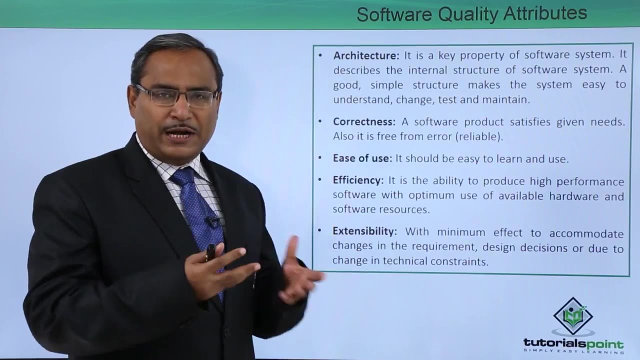 the key property of software system, So it describes the internal structure of the software system. A good, simple structure makes the system easy to understand: change, test, implement, maintenance, upgradations. So everything will be simple if you select the right architecture. 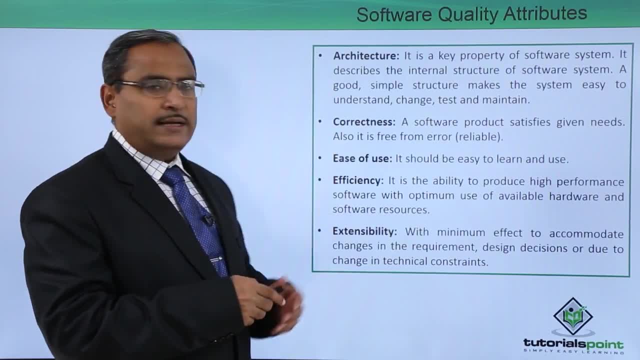 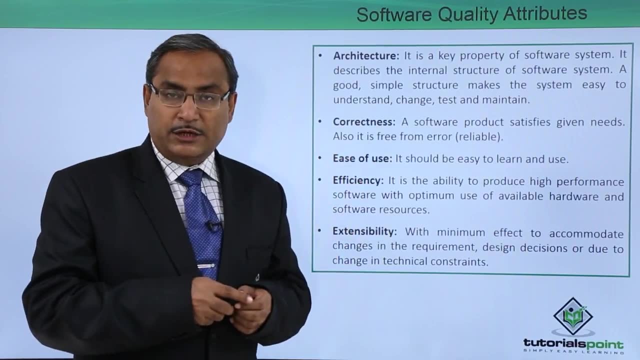 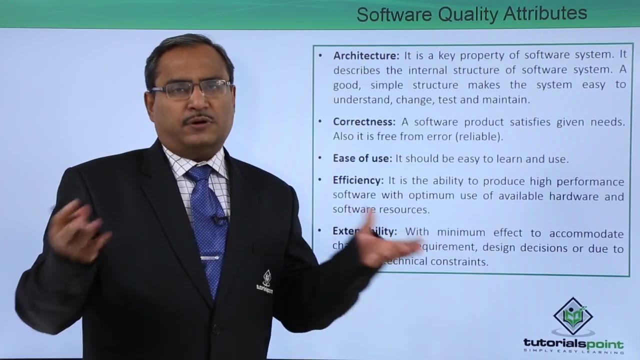 for the right software domain. Next one is the correctness. A software product satisfies given needs. Also it is free from errors and should be reliable. So let us suppose a client is demanding one software for some data processing, say for some numerical analysis oriented problems. 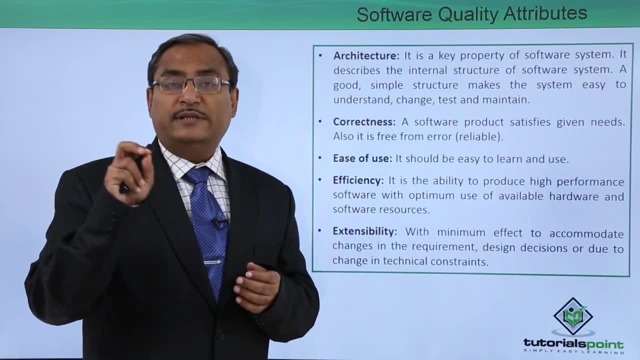 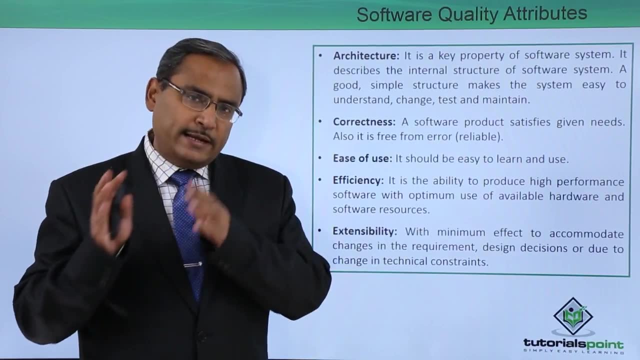 where he or she is requiring precision up to ten decimal places. So the precision of our output must be accurate to that ten decimal places. So the correctness and the reliability of the software should be up to that mark. Ease of use of the software in any protected environment can be survived Again. another: key property is where the standards are blurred. vetting and logging, manipulating the topics about the specific purposes cannot be avoided. You will also need to identify melhor world trends, know-how, marketing, universities, but problem solving and software major fields are also important to consider that, taking into account that solid languages can raise having any questions. 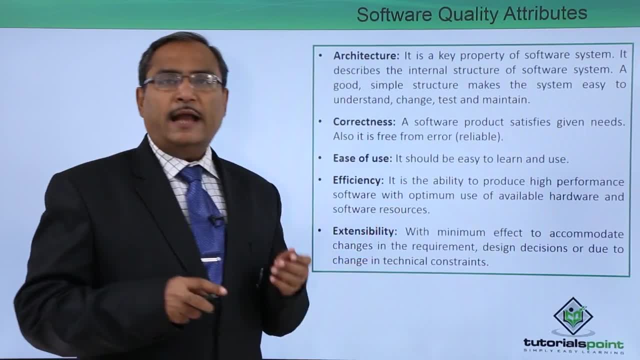 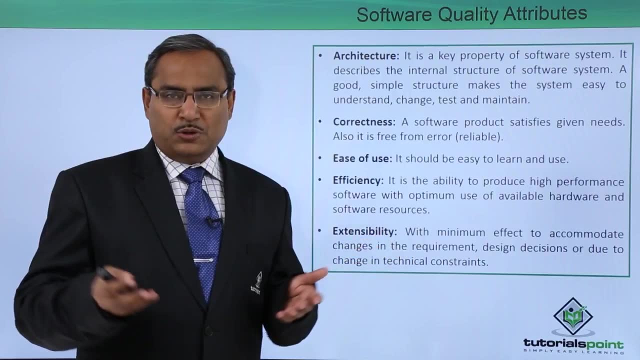 in a GAAS system. it also gem in such a way such as figuring between the basic case scene progress of use. it should be easy to learn and use. If you can make your software user friendly, the software will be more popular, more sellable, more clients will be liking using that software. 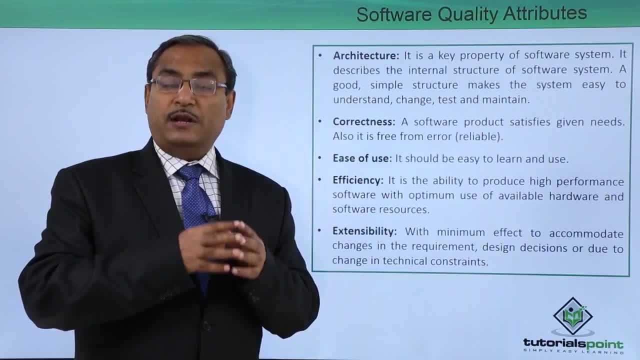 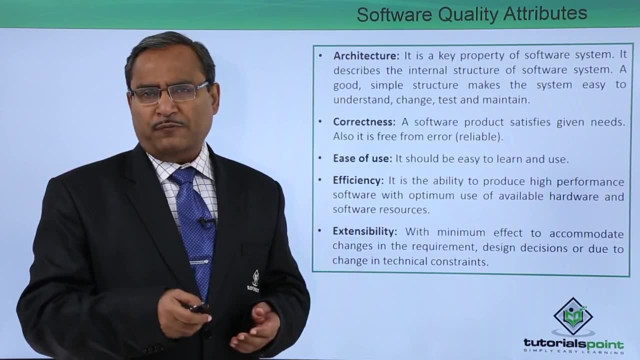 And if the software is really very much user friendly, if it is very much documented- the help files are very much documented- then the user may not be requiring a training to operate with the software. So that is why the software should be ease of use, easy to. 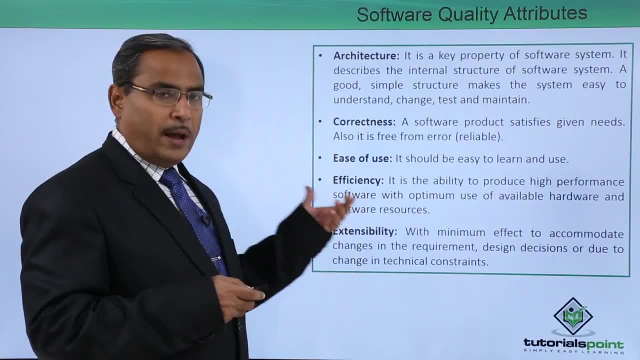 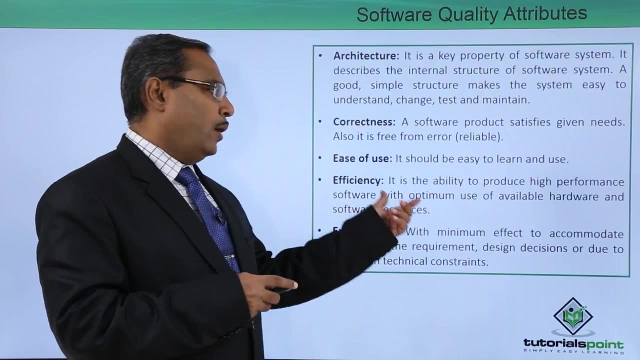 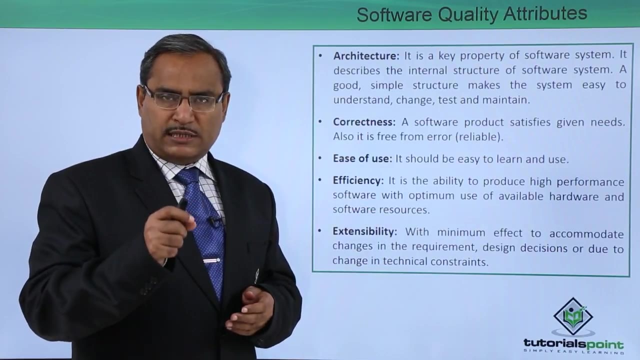 use and to learn and also to know about the software operations. Efficiency: it is the ability to produce high performance software with optimum use of available hardware and software resources. So if we can execute a process, if you can execute a thread, if you can execute one software with optimum software resources and hardware. 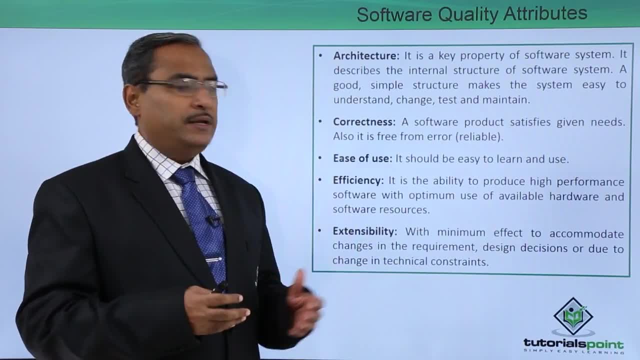 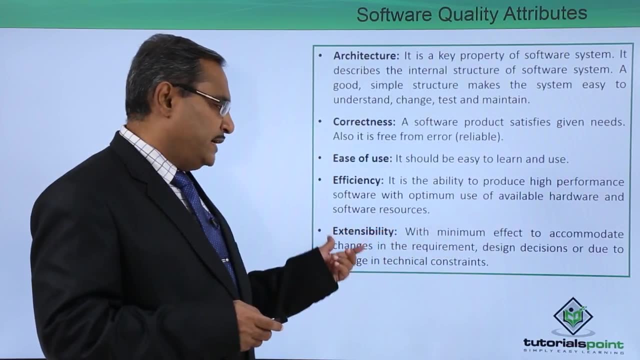 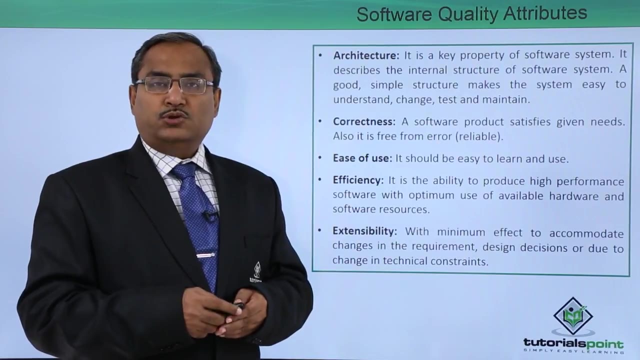 resources, then obviously you can say that this very software is very much efficient: Efficiency, Extensibility when minimum effect to accommodate changes in the requirements, design decisions and due to change in the technical constraints. So change requests will be coming from the 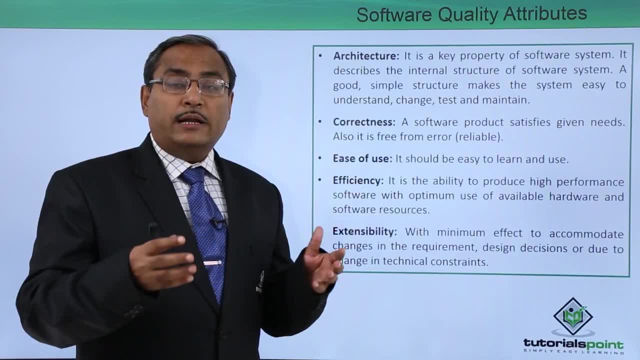 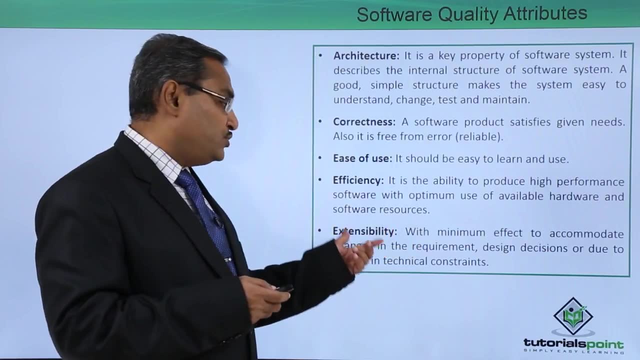 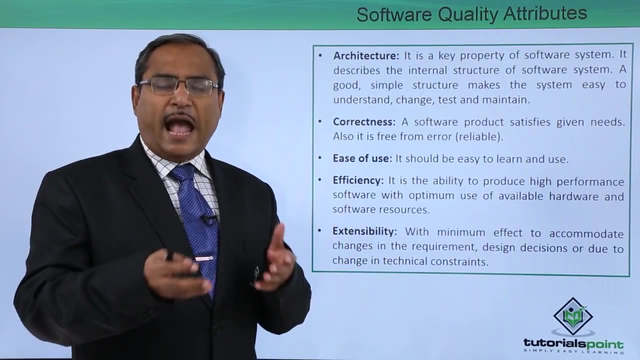 client. Different types of hardware and software, changes will be there. So that is why if our software is capable to accommodate those changes in the requirements in the design and due to some change in the technical constraints, If it can be accommodated accordingly easily, then obviously we can say that extensibility. 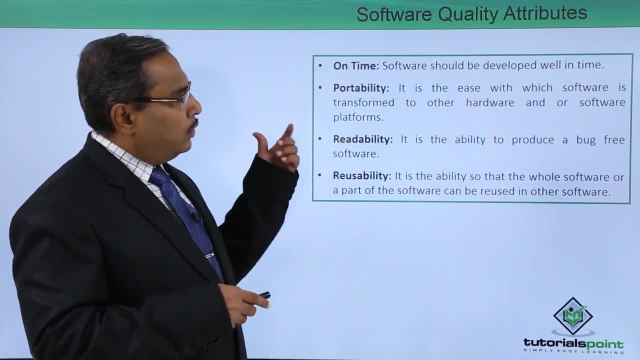 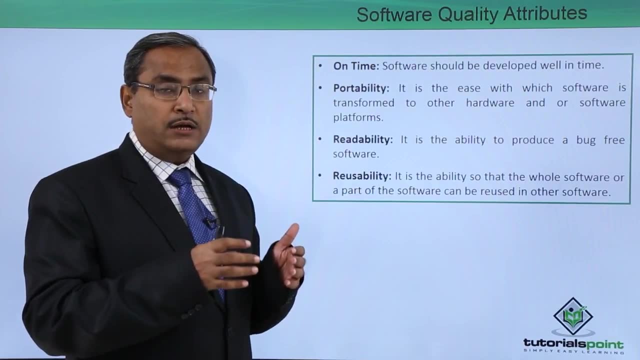 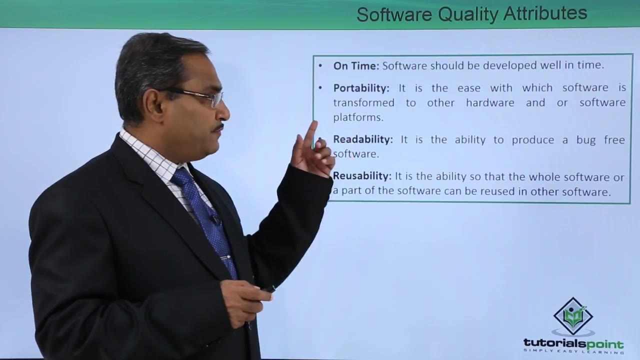 of the software is up to the mark On time. a software should be developed well in time, So it should be maintaining. the development should be done within the deadline. Portability: it is ease with which software is transformed to other hardware or to other. 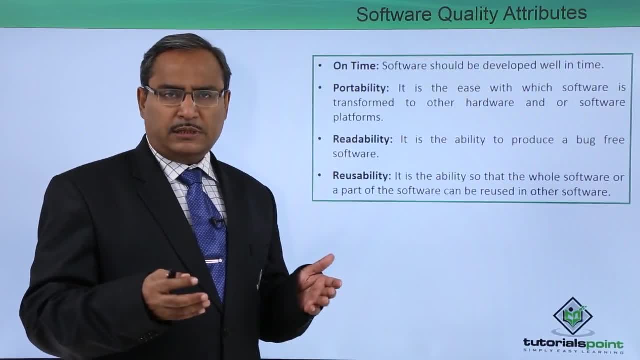 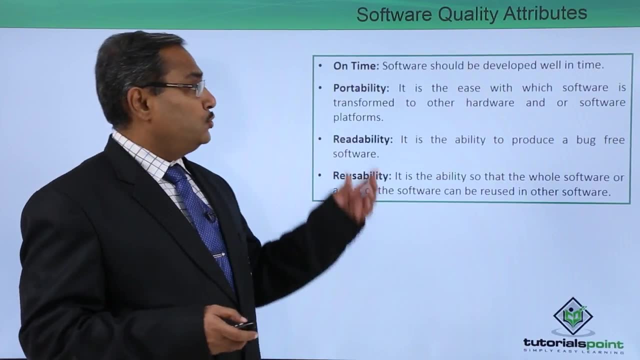 software platform. So what is the portability? What is the platform? Platform is nothing but the respective operating system and the hardware parts, the architecture of the machine. So that is why, if it is, if it is portable, so whether the portability is good enough or not, that means whether it can move from. 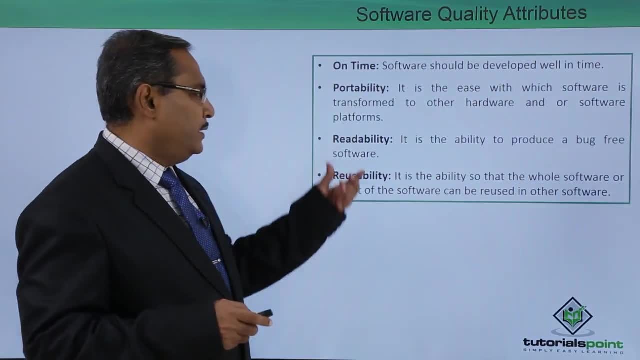 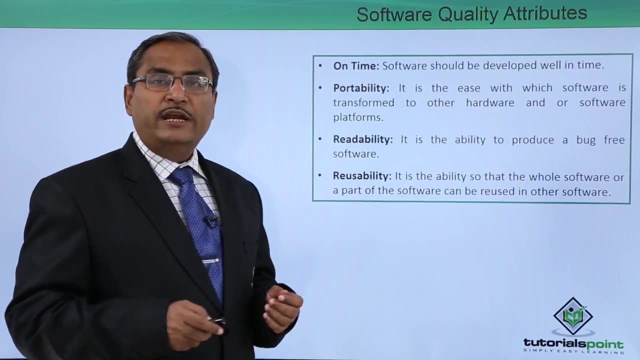 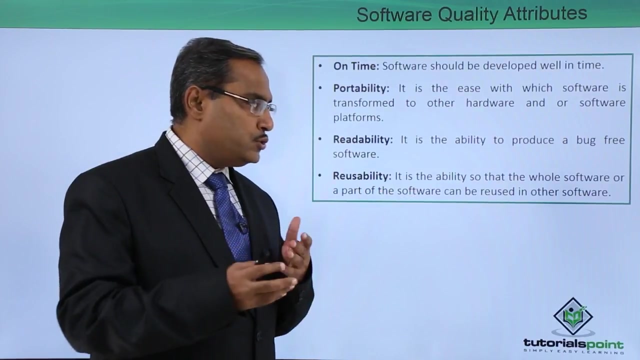 it can be transformed from one platform to another platform Readability: it is the ability to produce a bug free software. Next one is the reusability: It is the ability So that the whole software Readability, The whole software or a part of the software can be reused in another software, So that 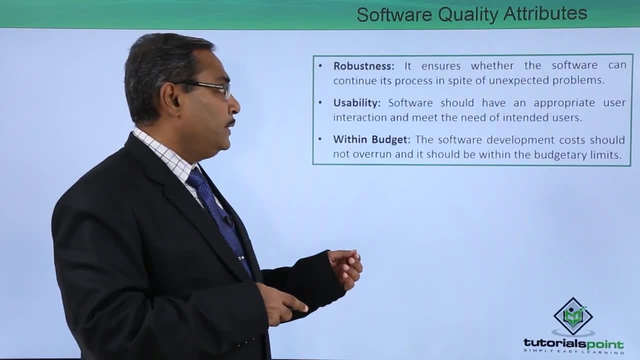 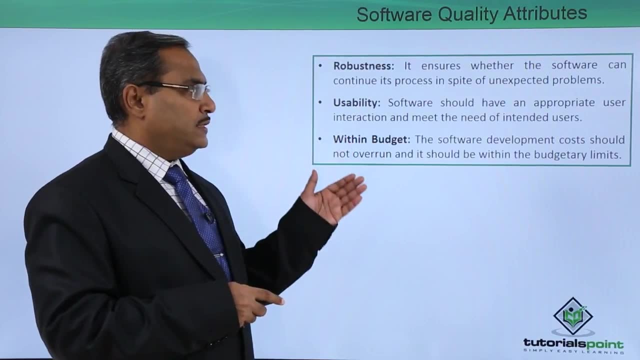 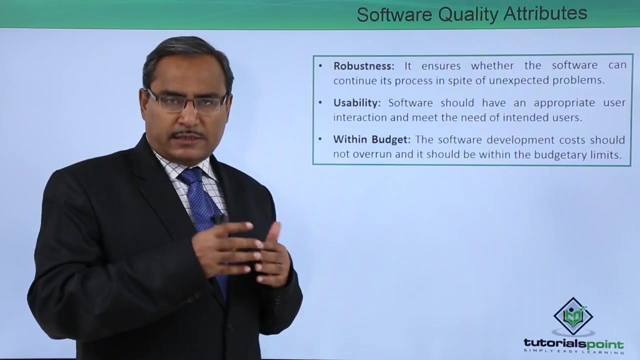 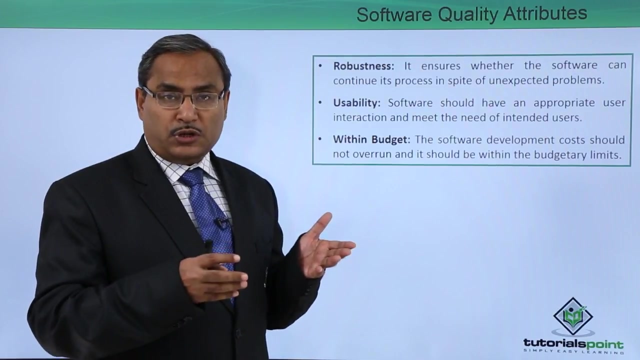 is known as the reusability property. Next one is the robustness. It ensures whether the software can continue its process in spite of unexpected problems. So that is a robust. that means the software is having some constraints or having some problems. but then also this: the software is executing in a continuous. 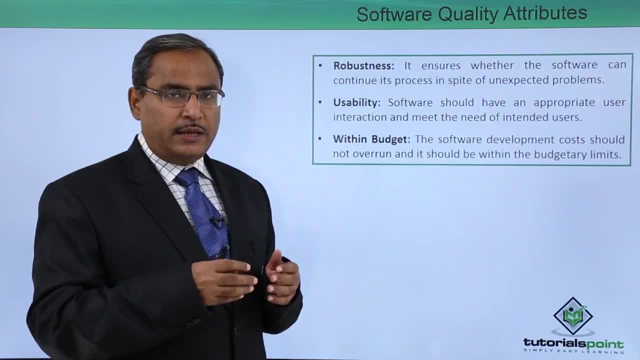 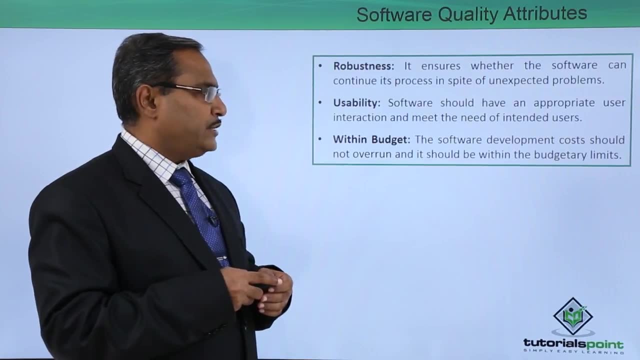 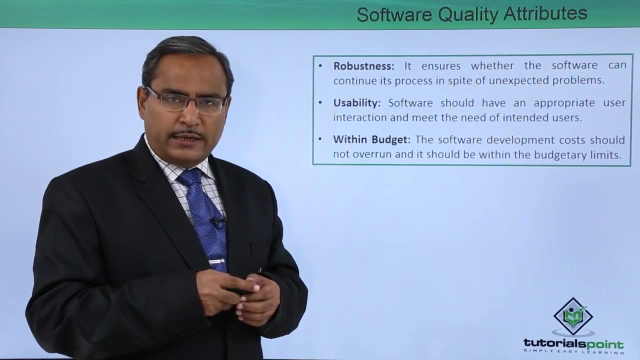 process. If it is so, then you can say that the software is having a good, robust feature. Next one is the usability. Software should have an appropriate user interaction and meet the need of intended users. So user interaction- there is a UI, user interface- should be good.